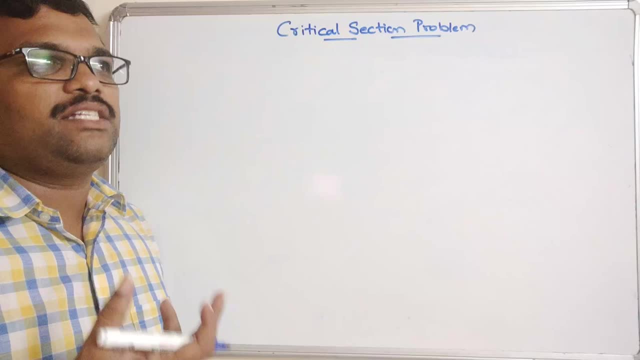 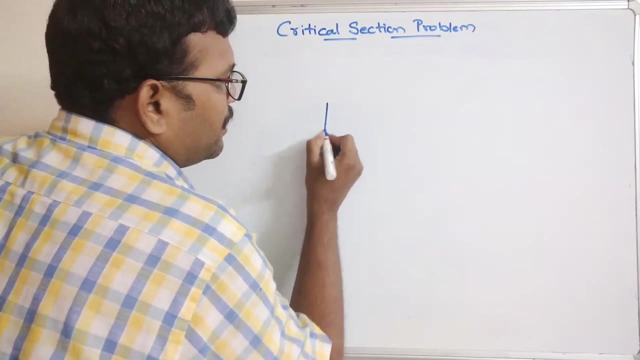 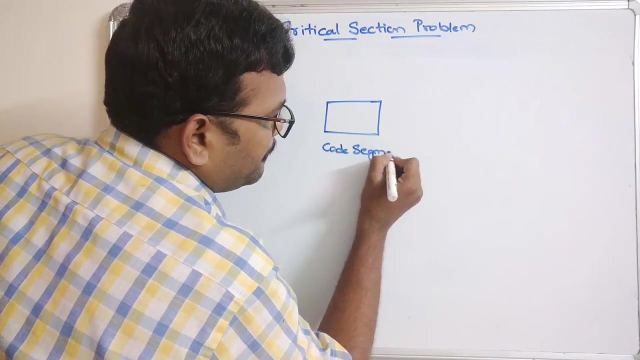 So, in order to avoid the race condition, such race condition, one should have a solution or one problem. is this critical section problem? So here, a critical section is a code segment. It is a code segment, So, which allows only one process to execute. 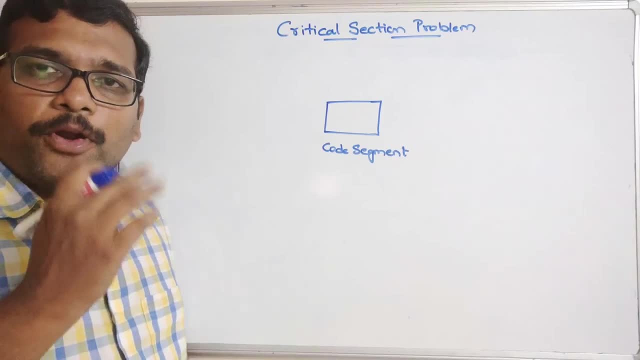 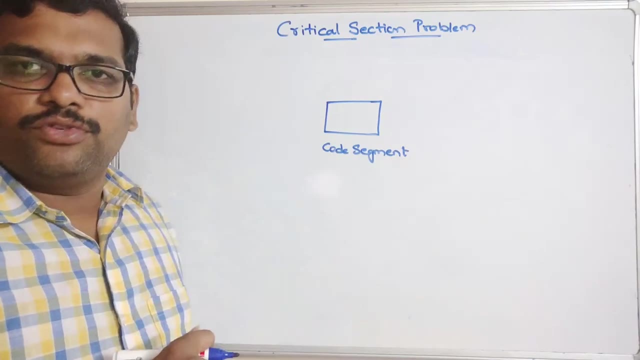 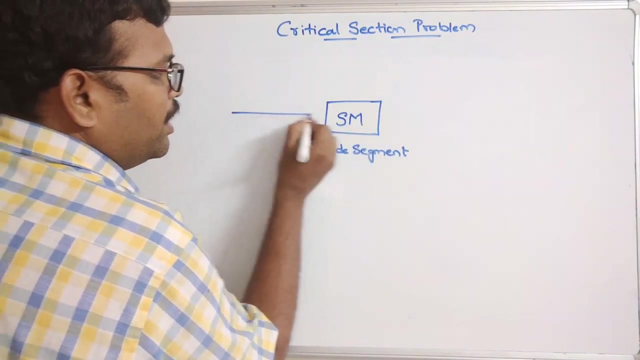 right? So if two process want to execute, if one process is being executed, the another process have to wait until the first process completes its execution, right? So The one process then has to wait for second process to execute. For that this is a shared memory. this is a shared memory. So if one process- see if there are. 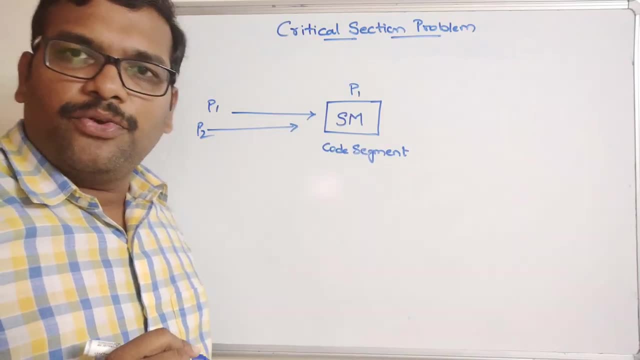 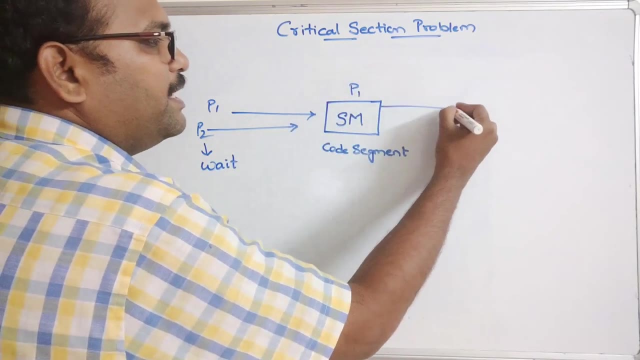 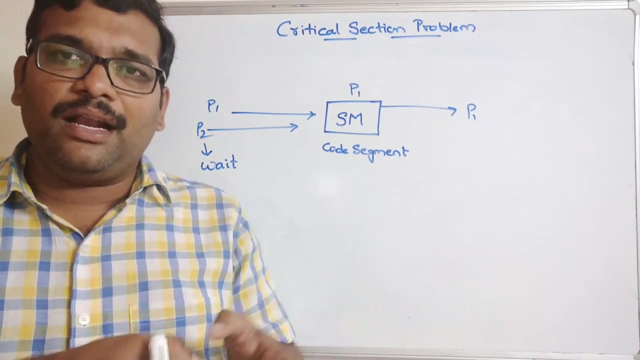 two processes. if one process is executing and the other process P2, have to wait until P 1 completes its execution. That means the P1, after completion of its execution, the P1, dealocates all the resources by bounded with the process, So in other words the single. 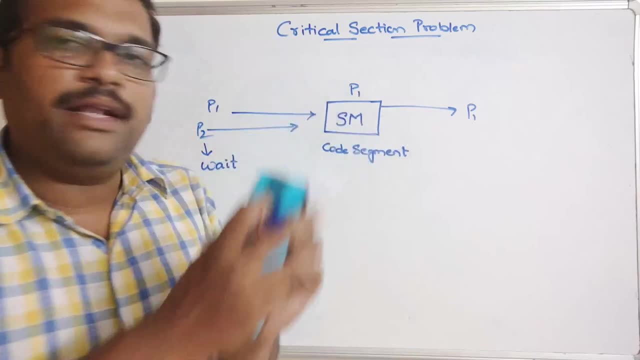 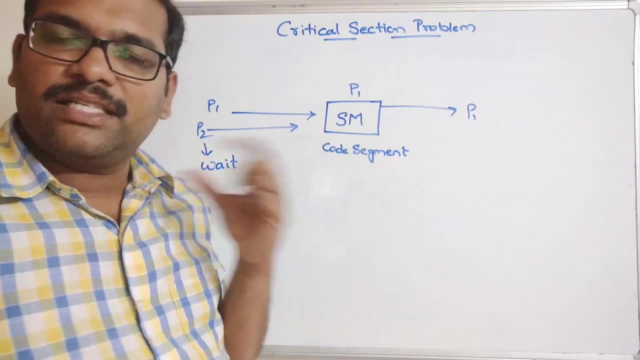 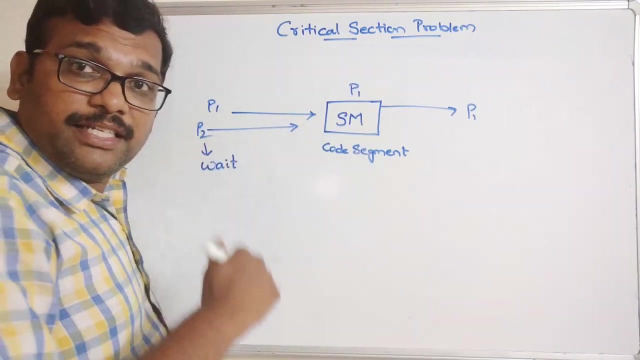 process and then only the P2 will be taking over the control of processor. so this type of thing we call it as a critical section problem, right, so here see, this is a code segment. as I have said, that critical section and this particular section is having the three things. one is the entry section, entry- 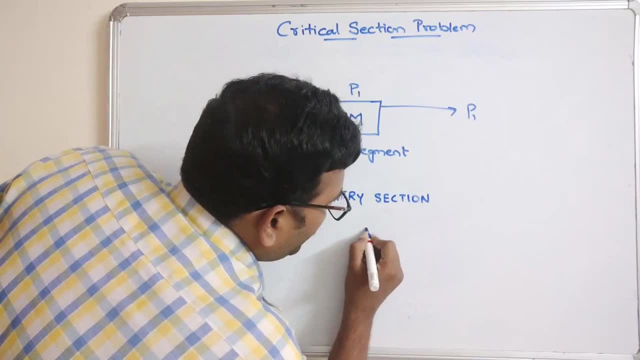 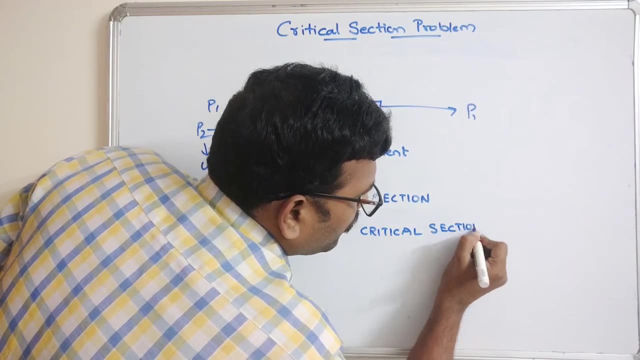 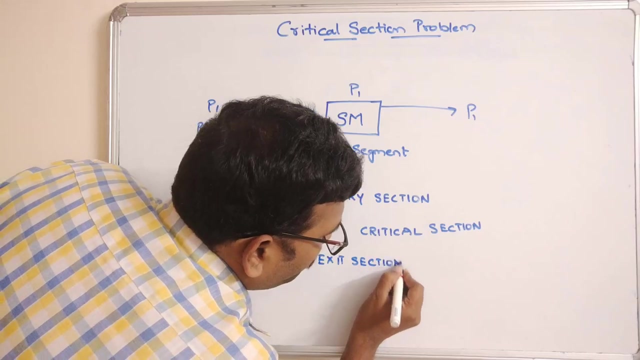 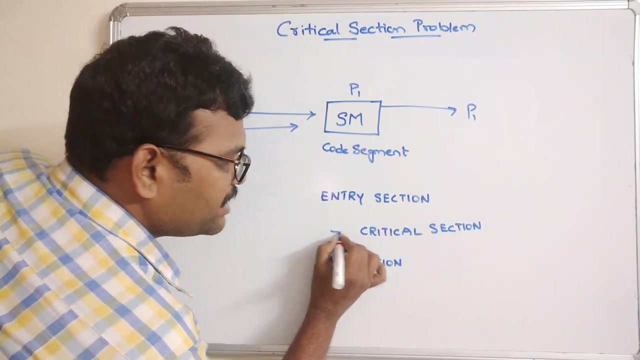 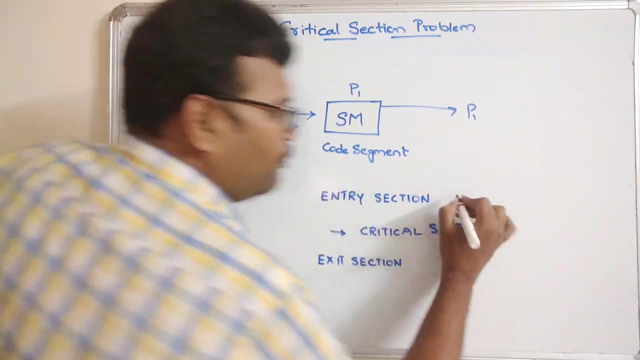 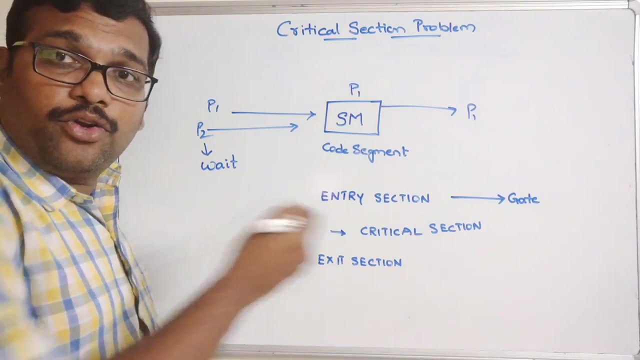 section and this is a critical section and this is an exit section. right entry section, critical section and exit section. so if one process is in a critical section, no other process will be allowed to execute right. so the entry section will be acting as a gate, a gate right to enter the process. 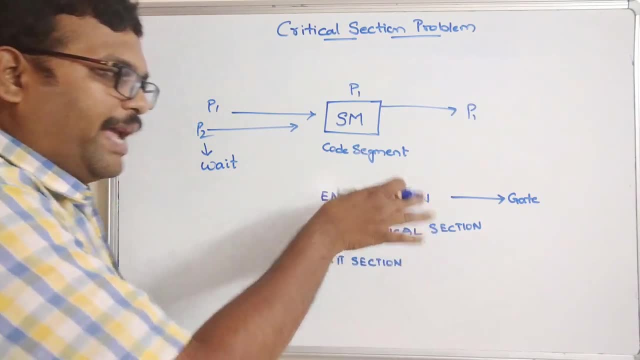 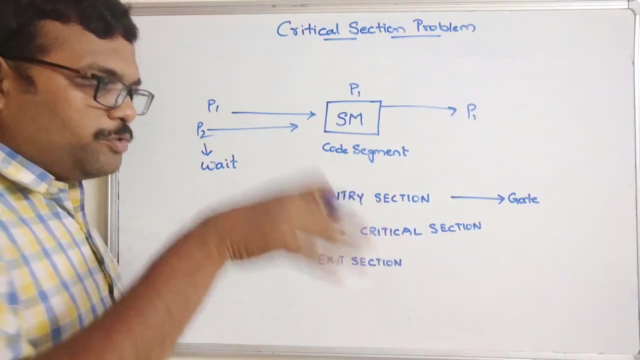 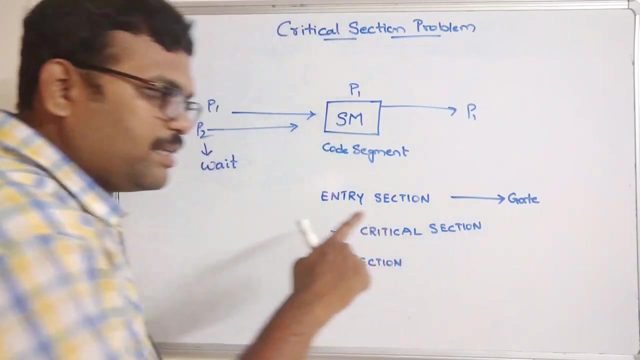 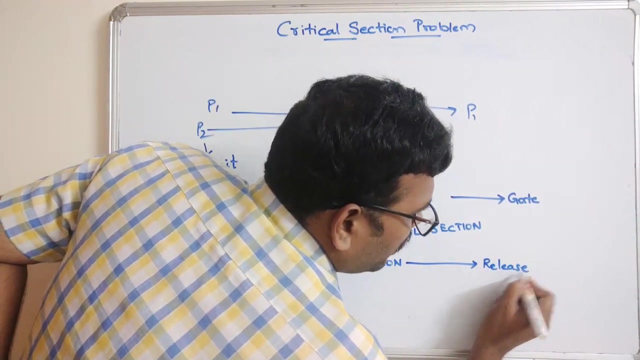 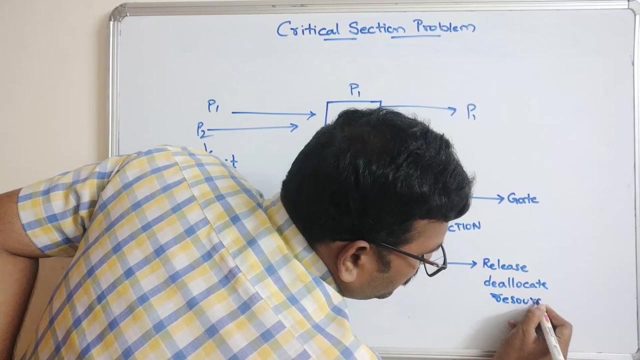 so one process enters into this critical section, the entry will be stopped for another process. right, if there are any other process wants to get executed, so that those process will be halted or waited by this entry section. and whenever a process completes its execution immediately, the exit section will release, release or deallocate resources, resources bounded with that particular. 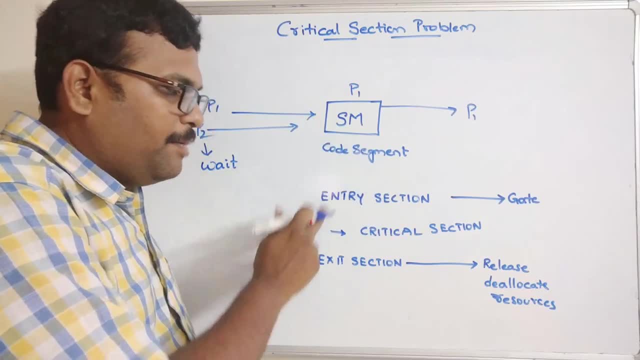 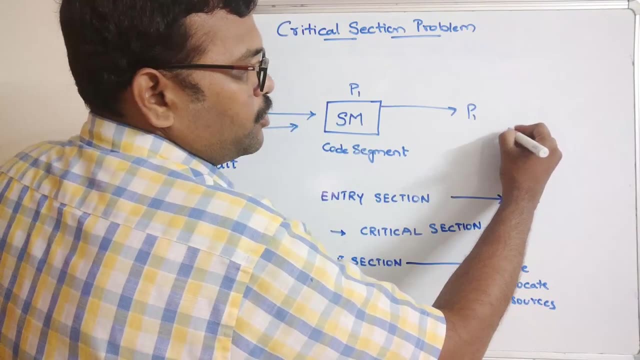 process, then only the entry section will enter. I mean will allow the another process to get enter into the critical section. for example, let us take P1 and P2, so P1 and P2 are the two and P3, there are three processes. okay, three processes. they need to get executed. 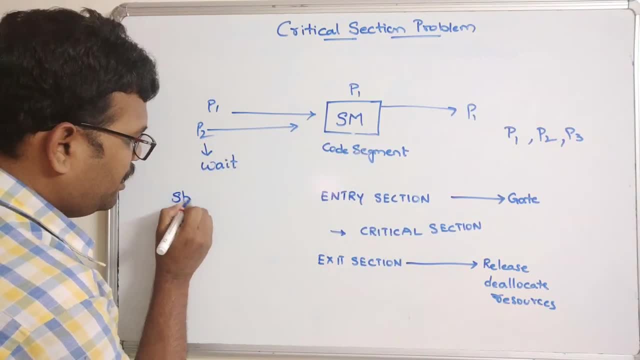 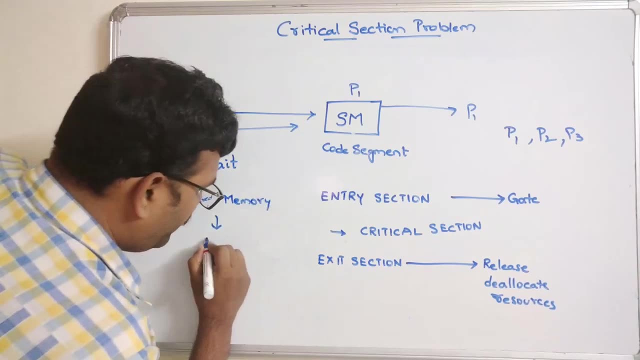 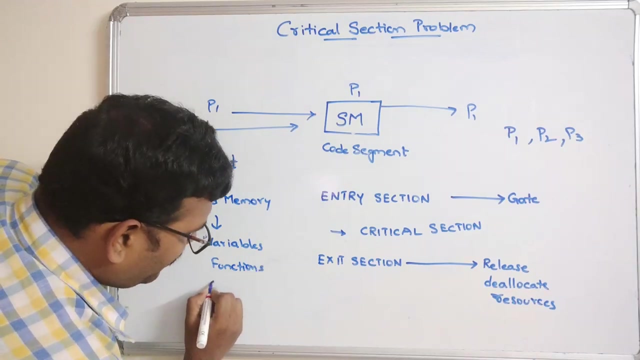 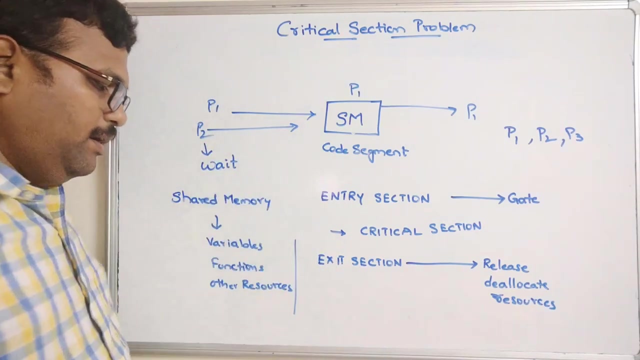 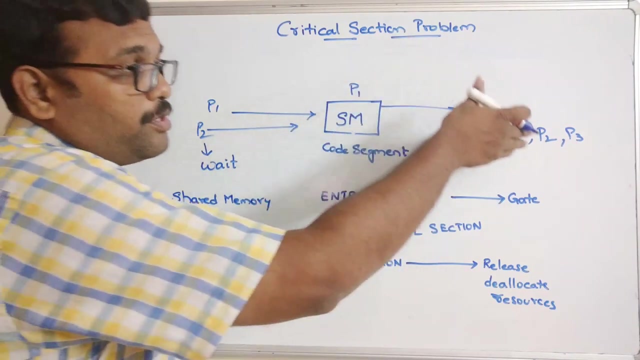 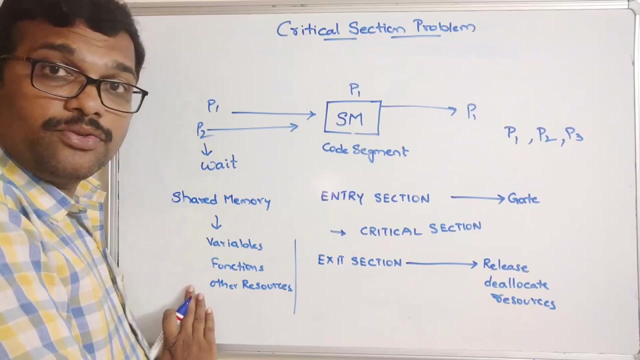 so here, the shared memory, shared memory. in this shared memory we can have variables, functions and any other resources, any other resources, right, any other resources. so if the process wants to be get executed, all the processes can access the shared memory: either they can access the variables, functions or other resources. 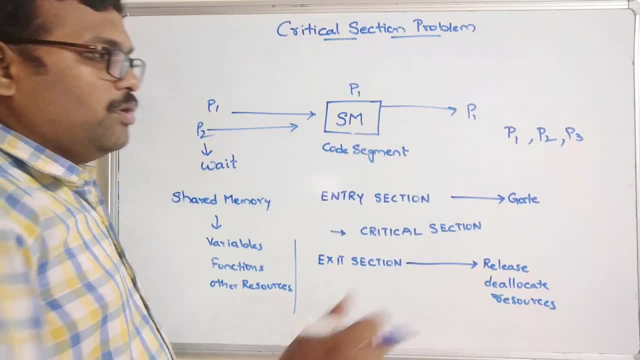 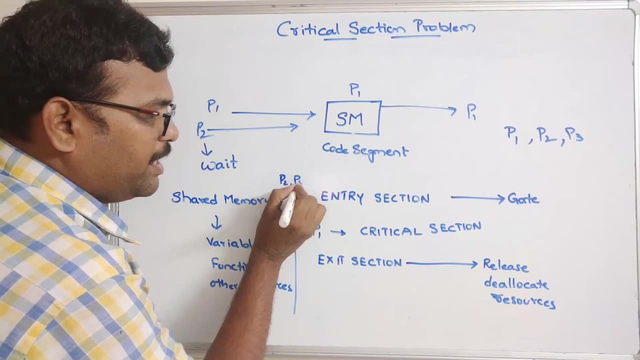 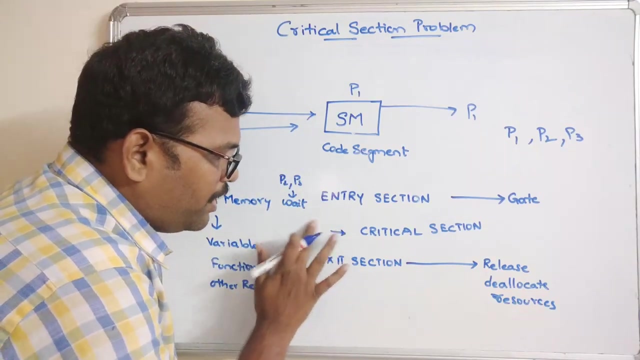 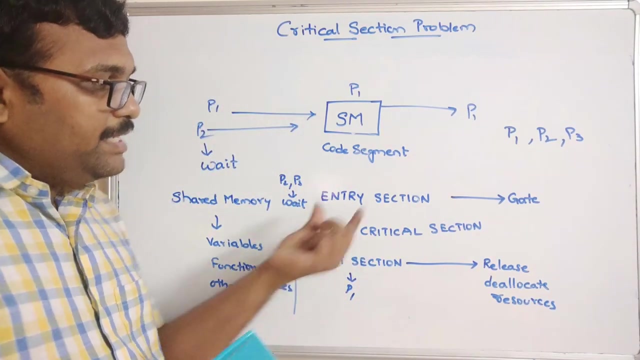 and all these are common to all the processes. so if P1 enters into this critical section, the P2 and P3, P2 and P3 will be in a waiting section, will be in a waiting section. so whenever the P1 get to the exit, then P2 will enter into the critical section. so entry: 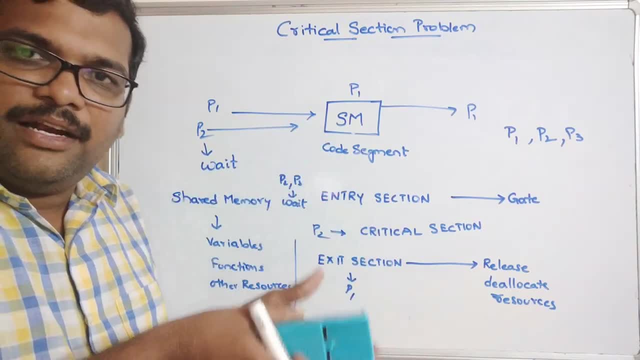 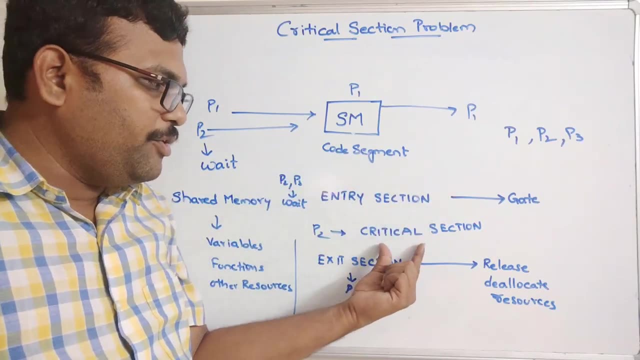 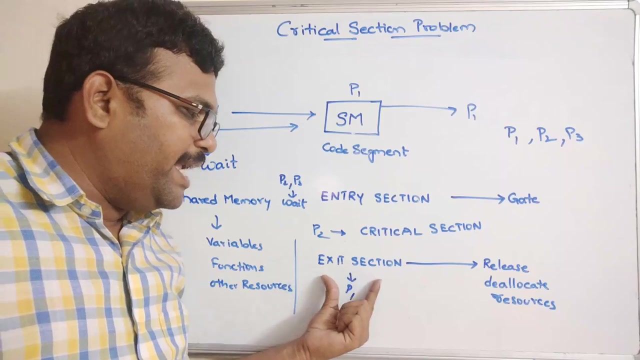 section is used to stop other processes to enter into the critical section until this critical section becomes free. so whenever the process is get executed in the critical section and whenever the process completes its execution, so the process will come to the exit section where all the resources and the shared memory will get executed. so 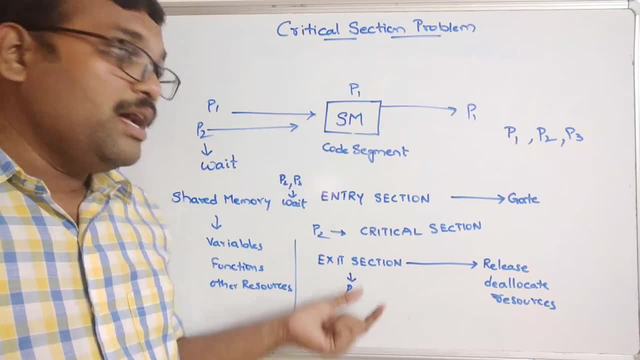 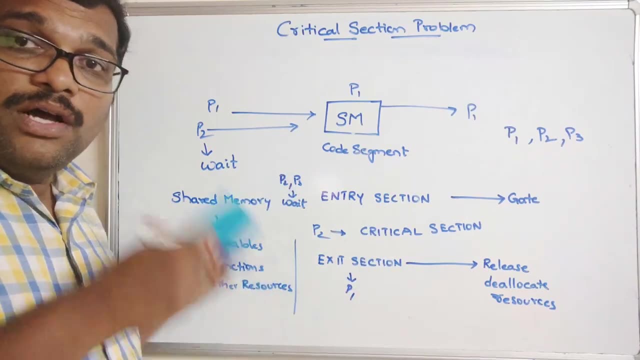 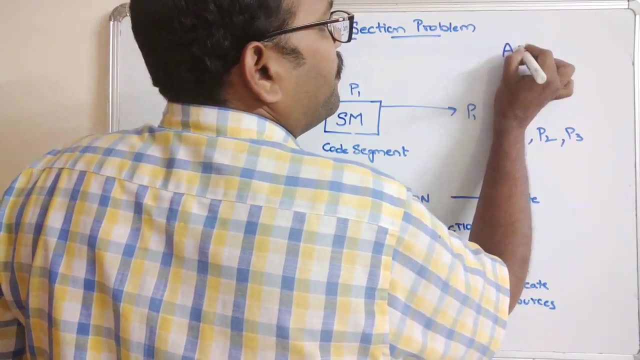 the shared memory will be released for that particular process, then only the another process will be allowed to enter into this critical section. so this is how the processes will be get executed. the best example for this problem is our ATM, so we all know about. 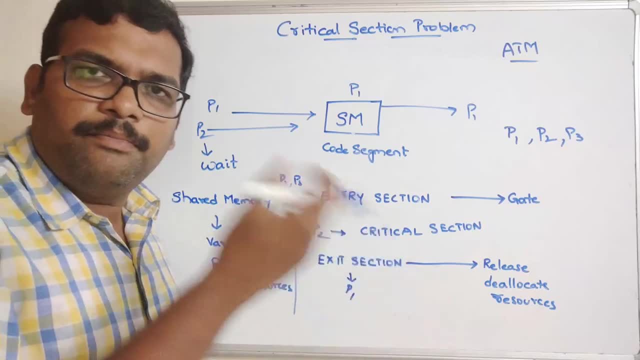 this ATM right. so any time we can go to the ATM machines and we can get the amount right. So at a time only one person can make the payment right. so any time we can go to the ATM machines and we can get the amount right. so at a time only one person can make. 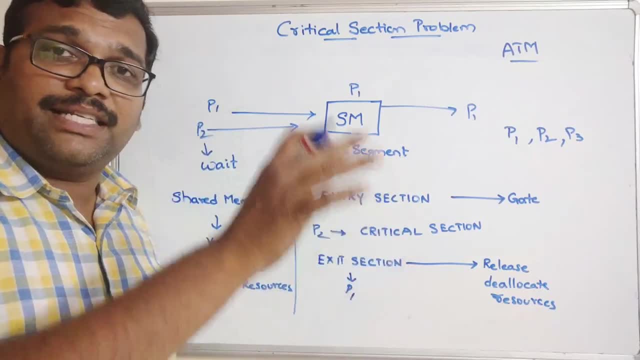 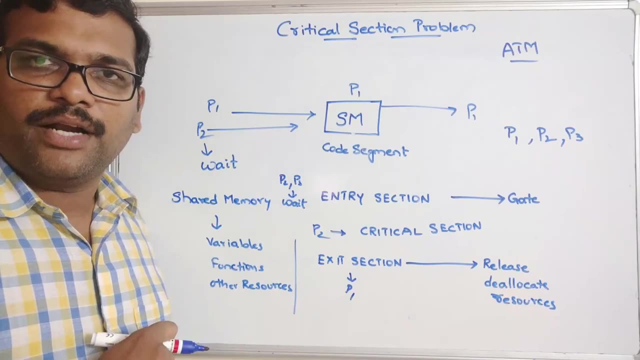 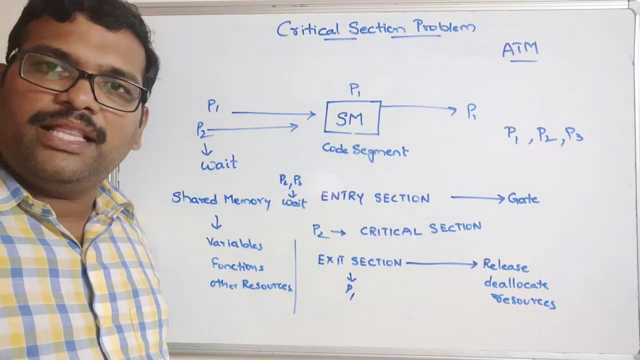 enter into the atm and once, if one person is availing the services, the another person have to wait until he or she completes its execution right. so once the person inside the atm have completed the services, so when he comes out, then only the second person will be allowed to. 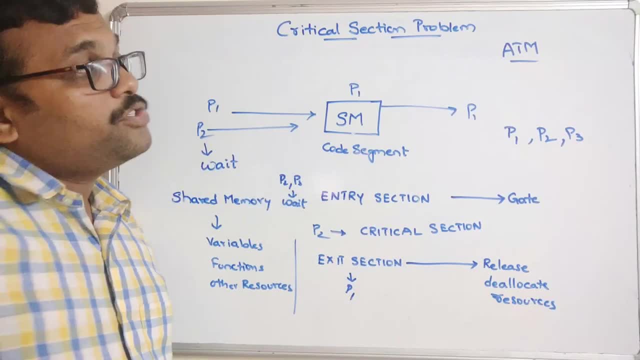 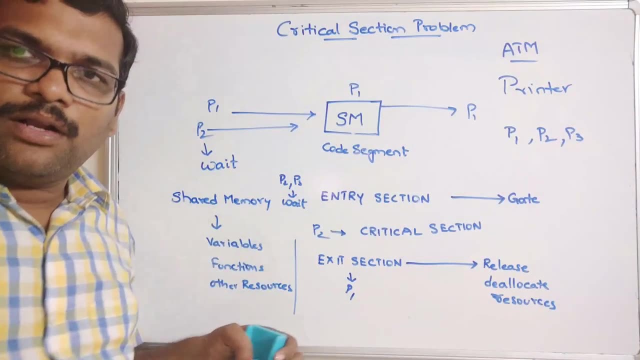 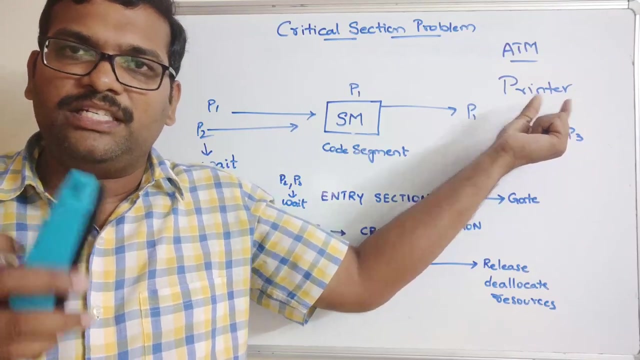 use the services in the atm machine right. so that is one example. another example: availing the printer service in a network. so if there is a network, we are having a lot of systems available in the network and we are having one printer, only one printer, which is shared among all the. 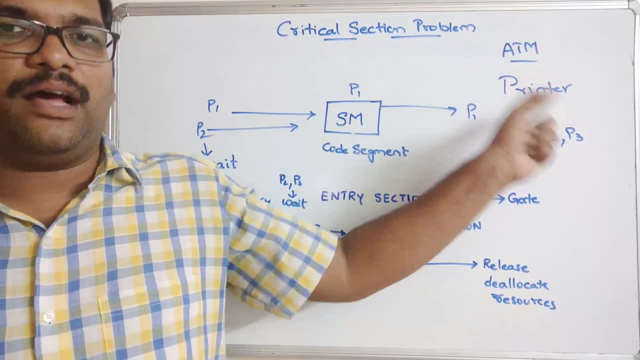 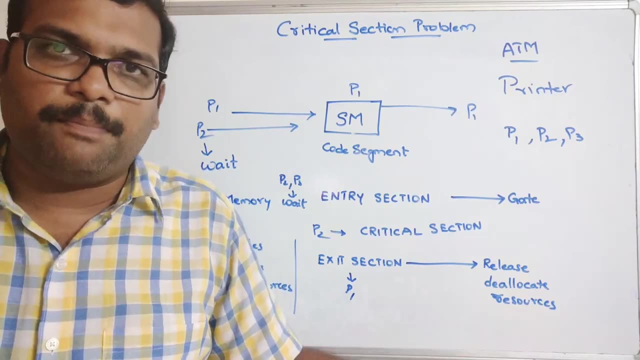 so at a time only one print can be done by the printer right. so if system 1 gives a print and at the same time if system 2 also gives the print, system 2 will be in the waiting state until the system 1 prints. i mean, whatever the job. 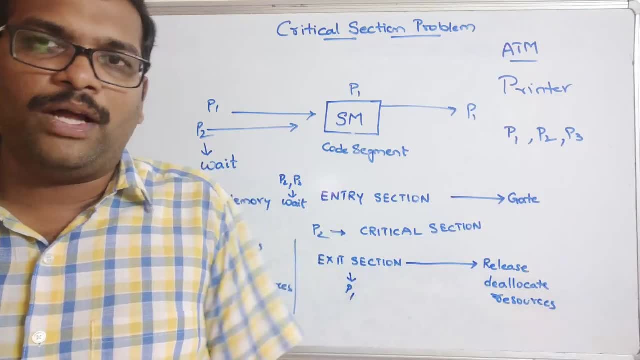 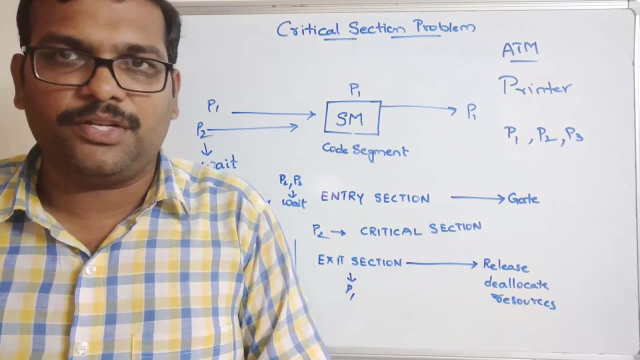 gives the system 2 gives the job- i mean whatever the job- gives the Hop into the system 2, so given by the system 1, completes its execution. so once the task given by the system 1 has been completed, then system 2 process will be get executed. so this is the example that means at: 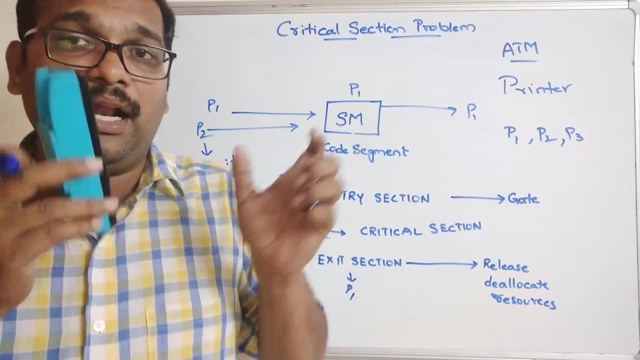 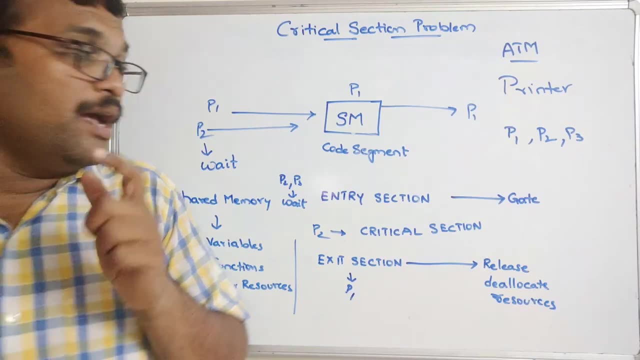 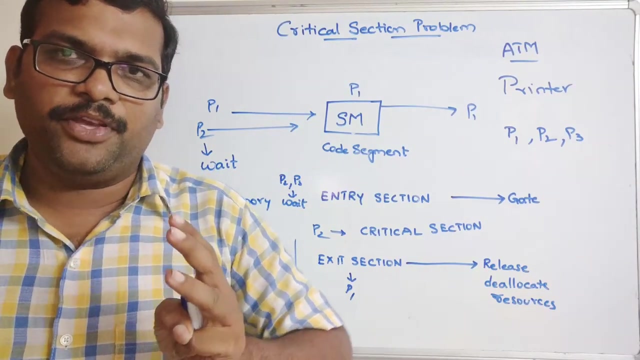 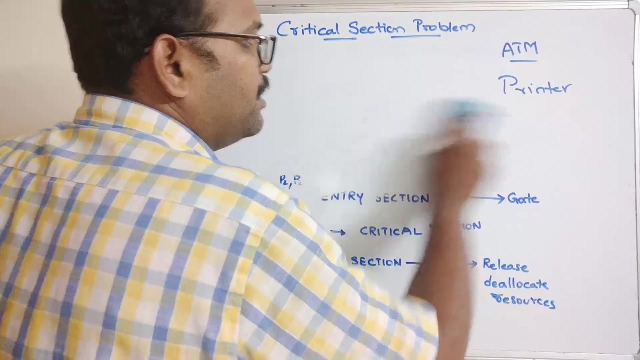 a time only one process can complete its execution and until it completes its execution, all the remaining processes will be in the waiting state. right now the solution is: the process should satisfy the three conditions in order to get in this critical section problem. so what are the three solution? i mean three conditions. so first condition is a mutual execution exclusion. 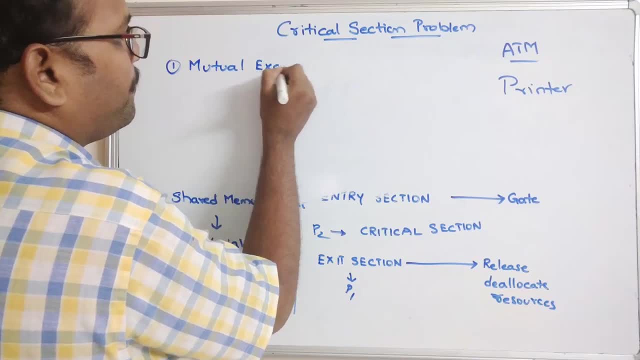 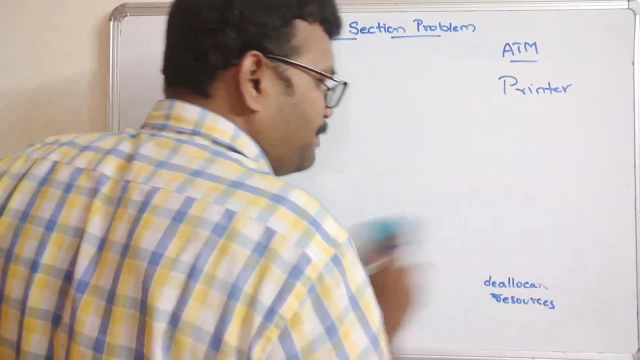 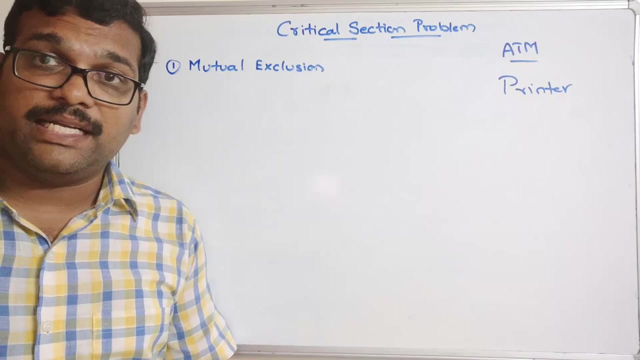 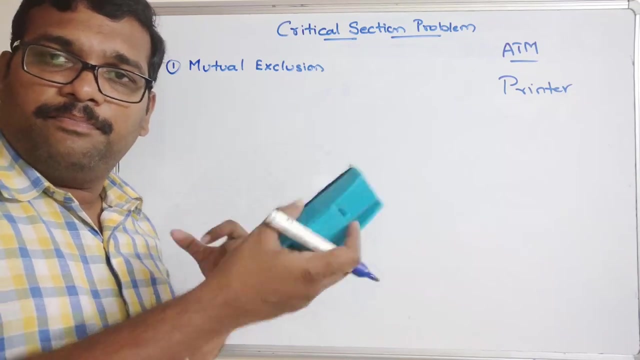 mutual exclusion. so every process should satisfy this. the the three concepts. so whenever these three conditions are being satisfied, that that mean there is a synchronization, so there will be no race condition. so in our previous example we have seen the two processes are having- i mean sharing- the same. 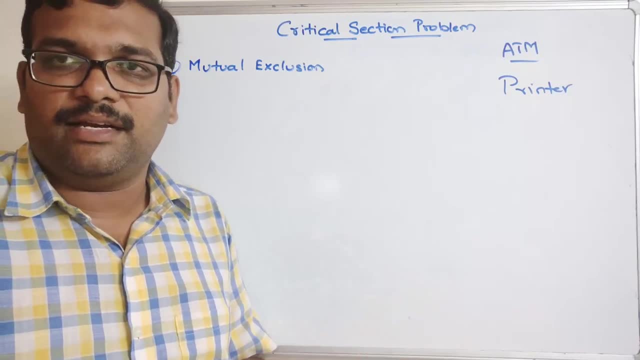 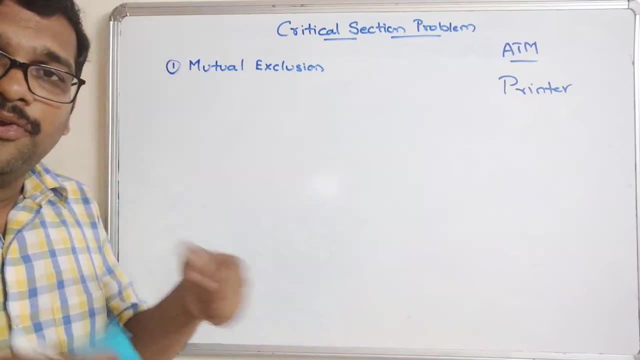 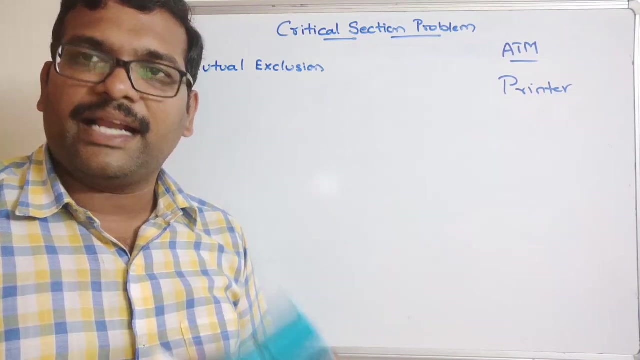 memory, so the data will be inconsistent. so we have seen some three instructions for producer and three instructions for consumer. so executing the instructions may give the inconsistent data right. so that is why we are getting some race conditions right. so here, if the process obeys these mutual 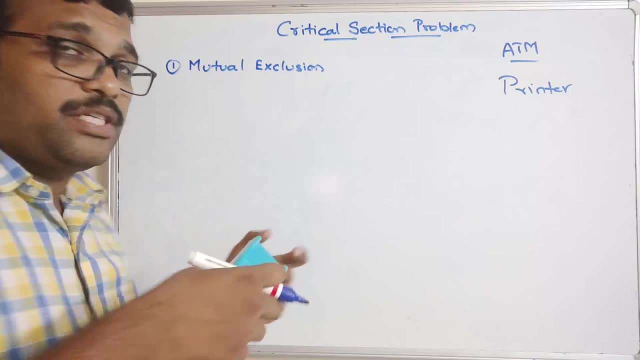 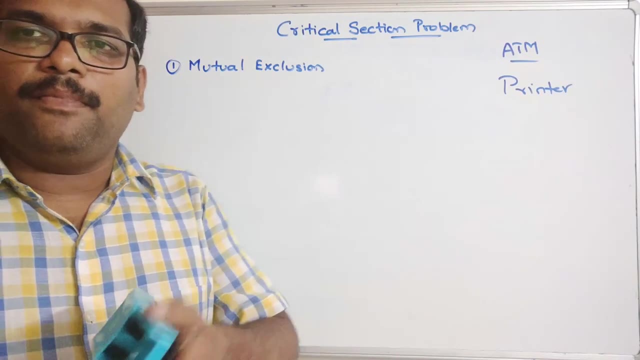 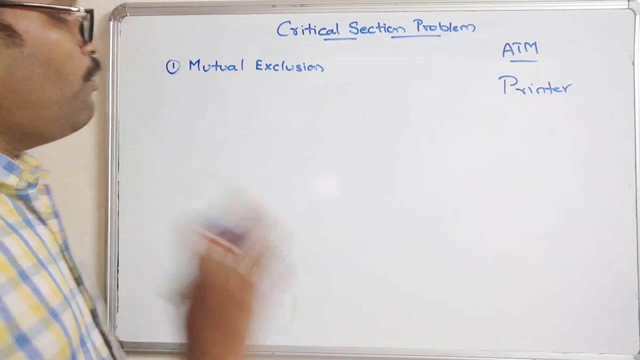 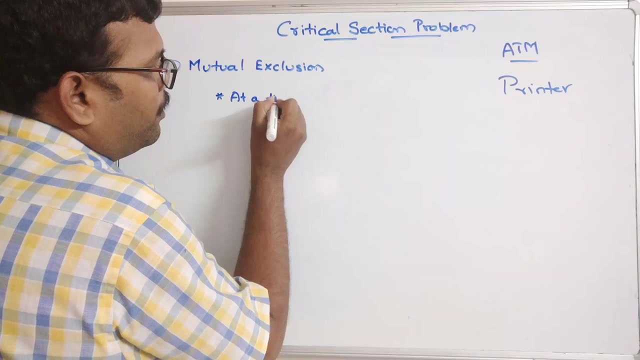 excuse exclusion and the remaining two process. that means that remaining two conditions like progress and bounded weight, so automatically there is a uh overcome of race condition. there will be no question of race condition. the data will be always consistent. so what is a mutual exclusion? so mutual exclusion means: so at a time, at a time, only one process. 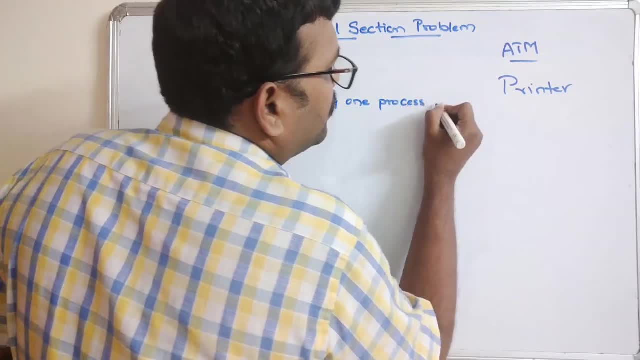 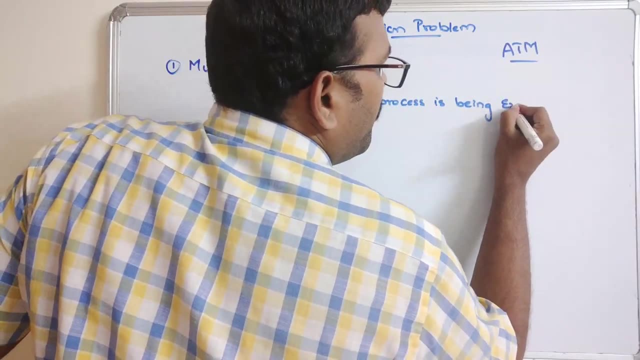 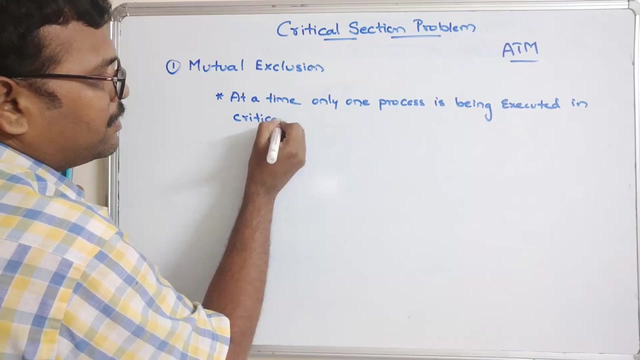 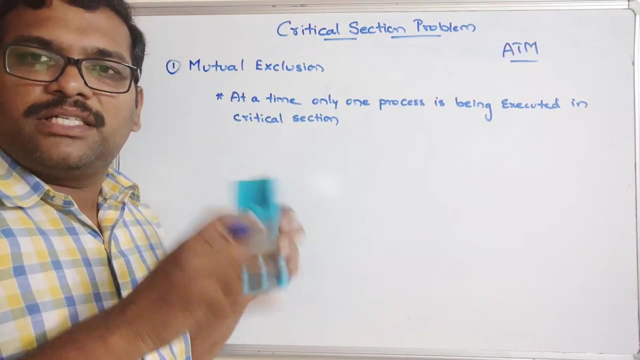 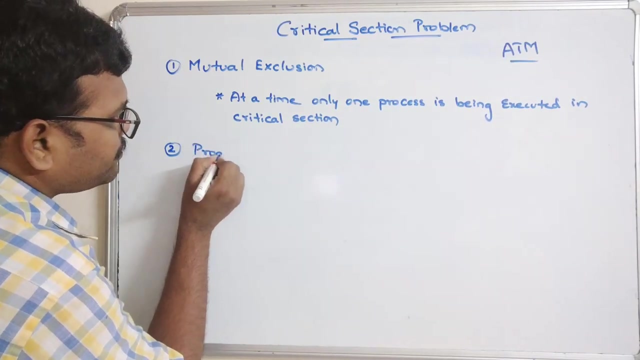 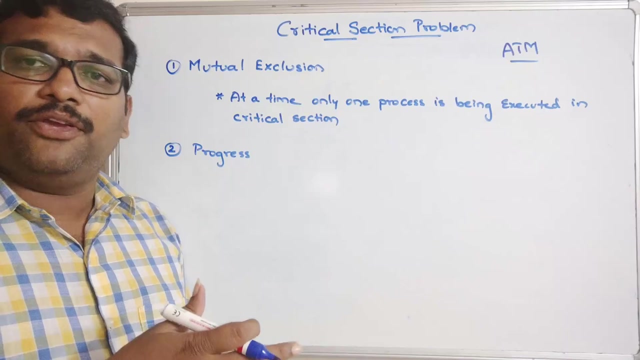 only one process is being executed in critical section, in critical section, right? so if one process is in the critical section, the other process have to wait. that is called a mutual exclusion. and the second condition: progress, progress. so progress means if any one of the process doesn't want to execute, uh, in the critical section, 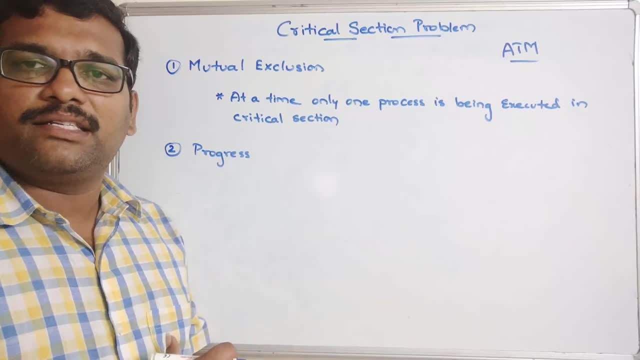 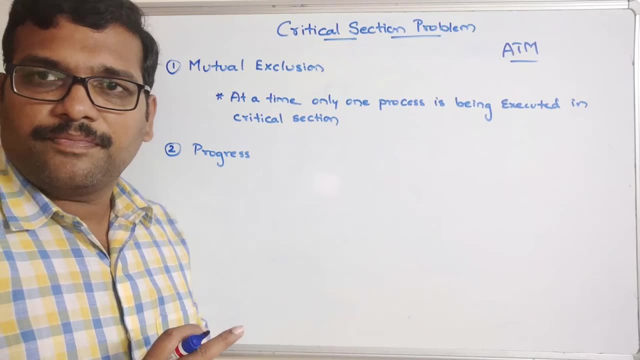 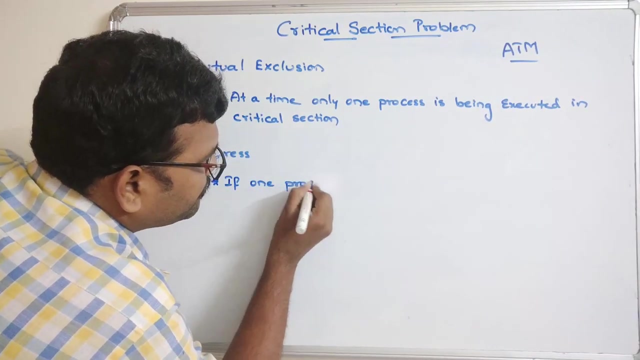 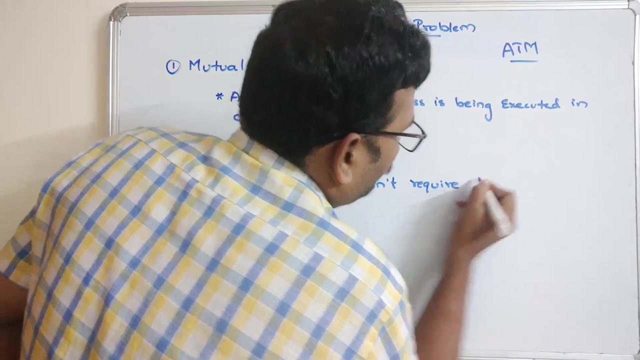 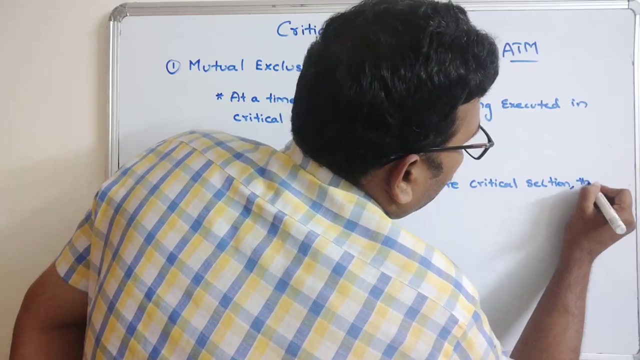 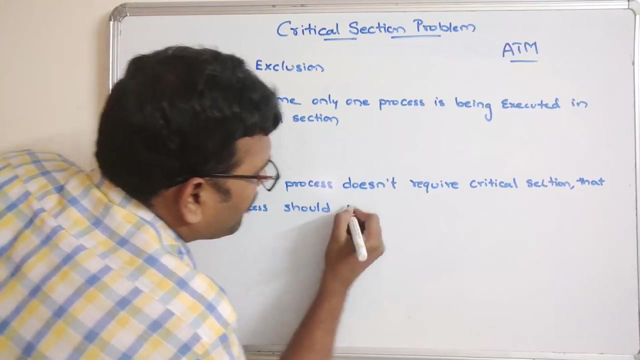 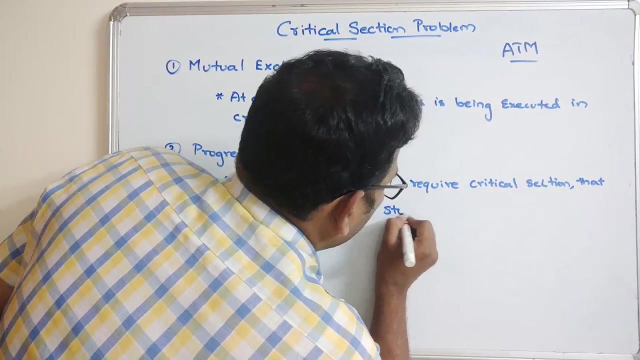 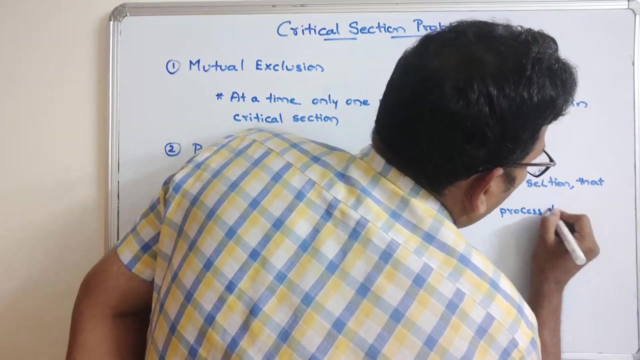 it have to allow other process to enter the critical section and uh, other process need to execute the process right, so that is called a progress. that is called a progress. so if one process doesn't require critical section, that process should not stop the other process to get executed. 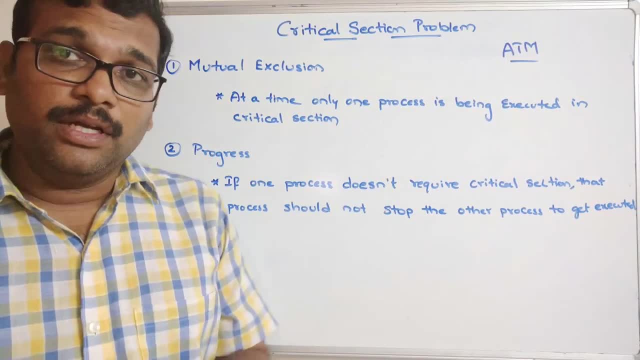 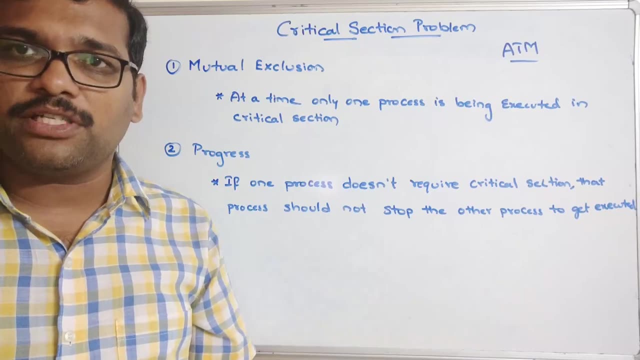 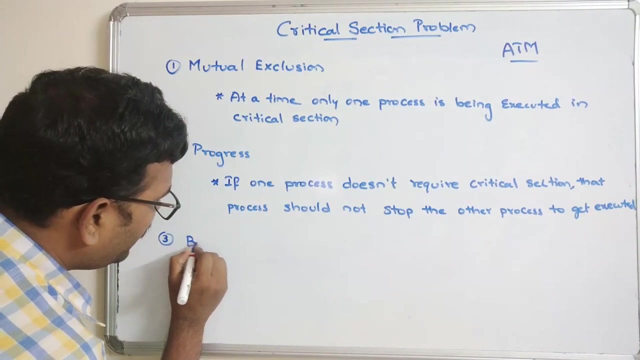 so if one process doesn't need the critical section, it should not stop the other process to take, uh, the control of this critical section right. so we have to allow other process to complete its execution right. and that is the second one and the third one, bounded weight. 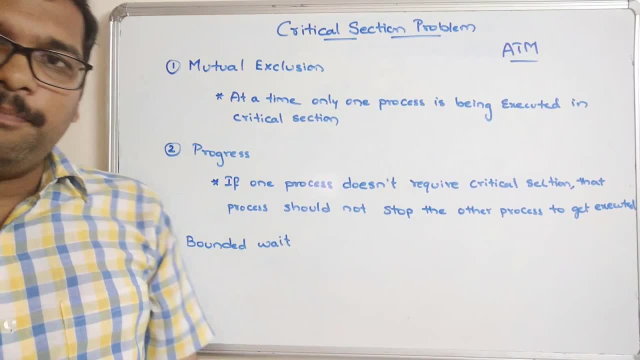 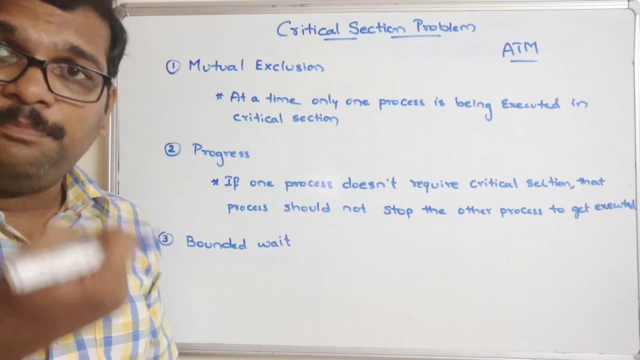 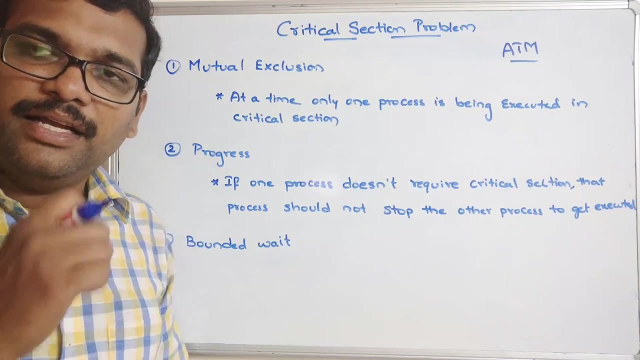 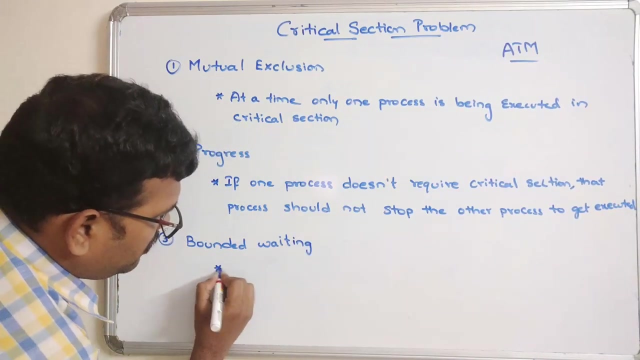 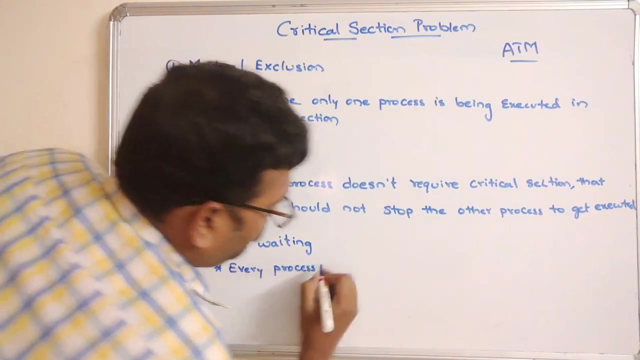 bounded weight. so actually this bounded weight means so every process should have some boundary of waiting time, right? so there must be some prediction. there should be some prediction how much time the process needs to be get completed, its execution right. so bounded waiting, so every process has to be completed. 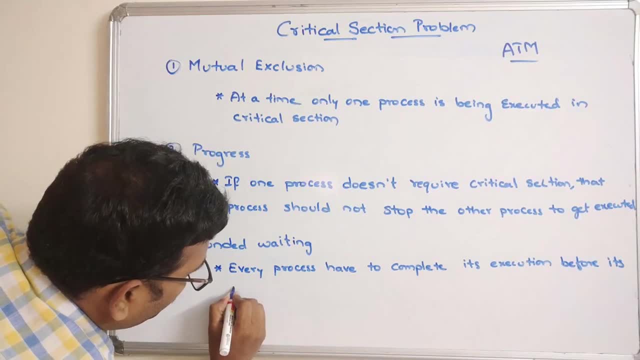 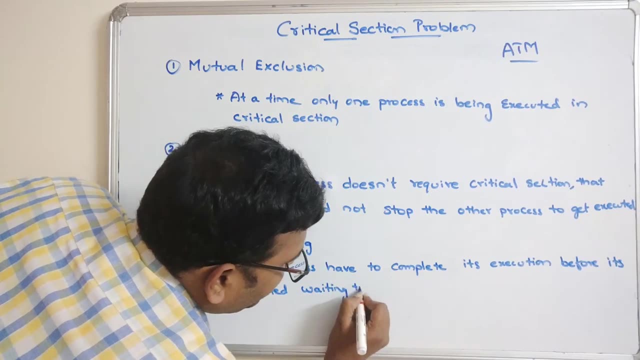 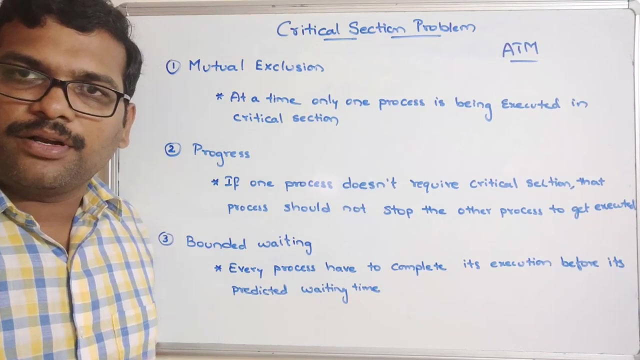 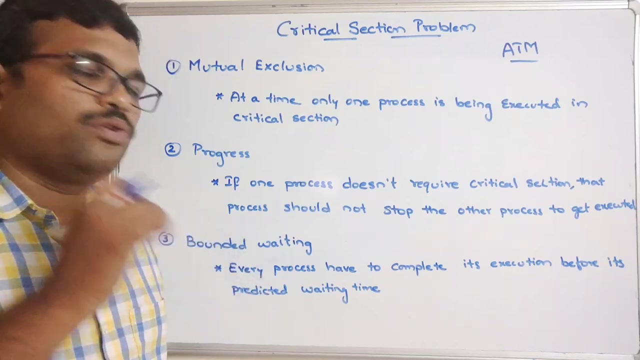 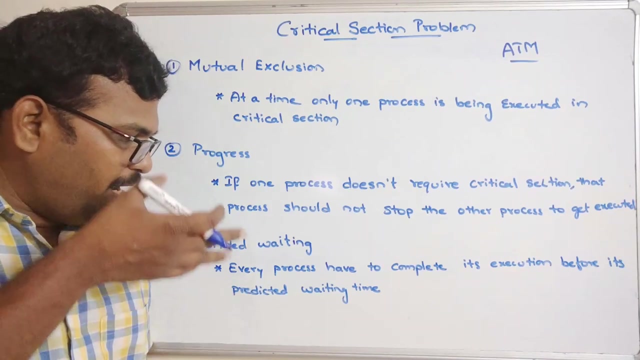 how to complete its execution before its predicted waiting time. waiting time so amount, I mean some sort of time to complete the execution right. so we have to predict that time waiting time right. so every process should complete its execution before its predicted waiting time, right. so this, mainly this condition. if any process face this condition, automatically. 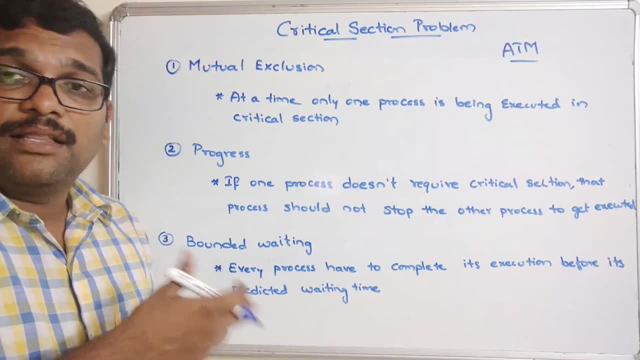 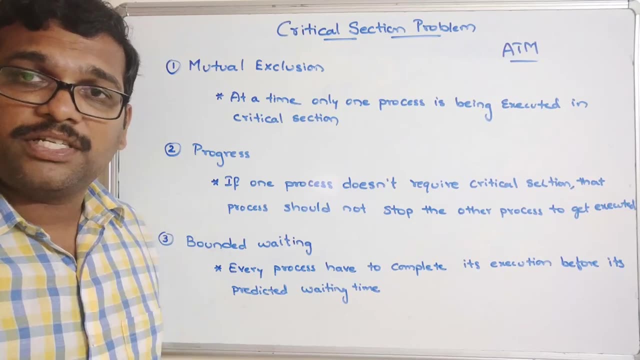 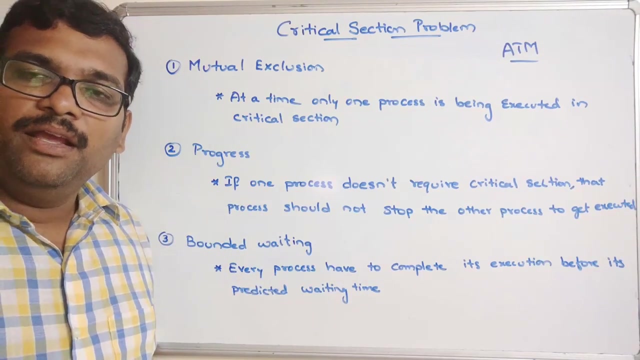 there will be becoming a starvation problem. that means the other process which is waiting for the critical section will be keep on waiting for the for its execution. so, whatever the process which is available in the critical section doesn't complete its execution, and still the remaining processes will be in a waiting state. so that should not happens. so after some amount of time, 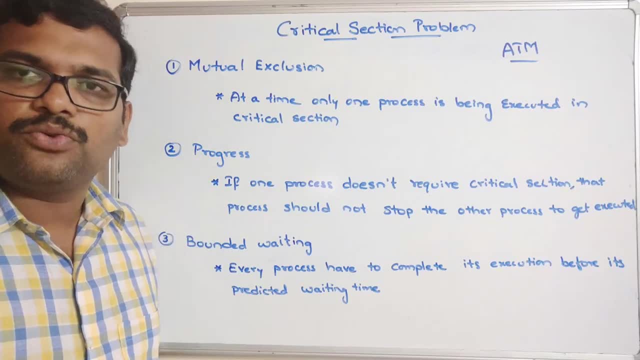 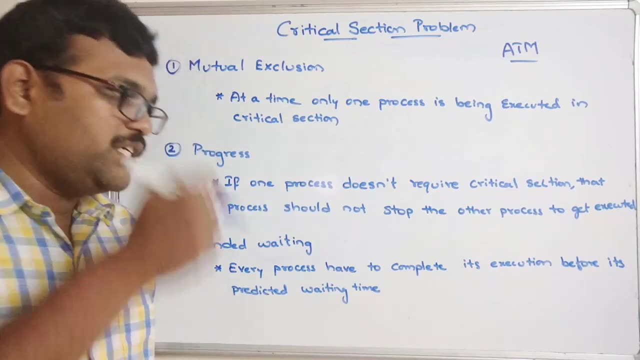 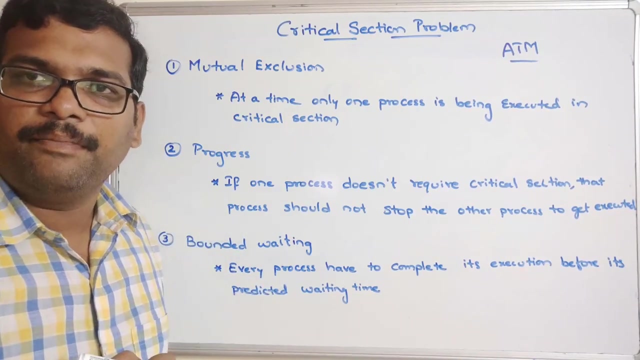 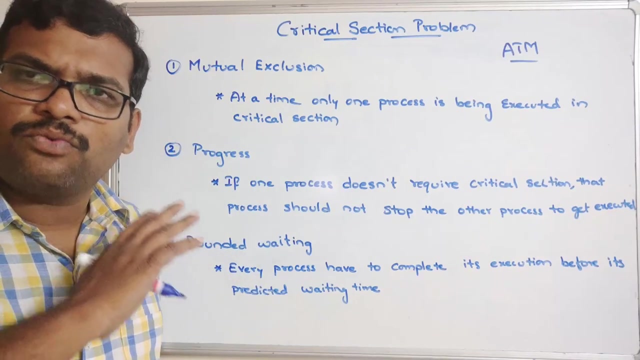 so the process should give the control to the another process to complete its execution. so there should be some limitation on waiting time. so the process which is availing the critical section should a complete its execution before that particular boundary of waiting time. So if any process satisfies all these three conditions, then there is no question of race. 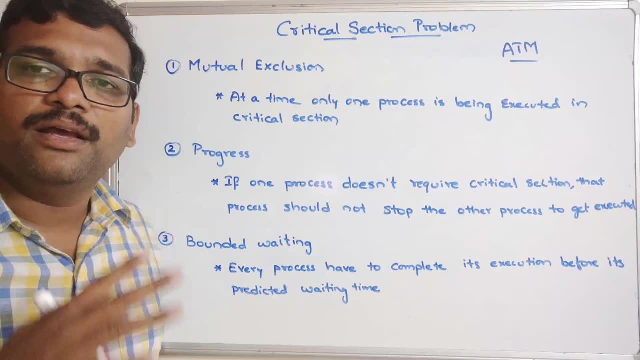 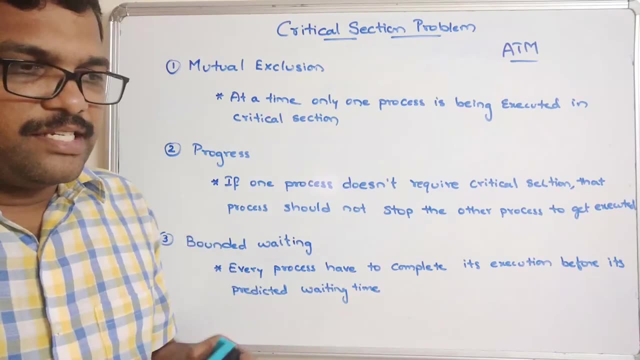 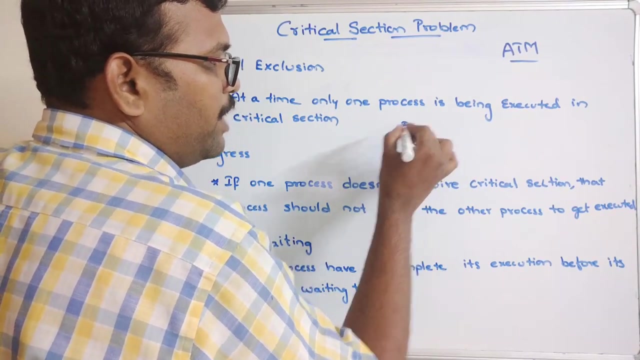 condition. So automatically, the process synchronization will be possible, right, And the data will also be consistent. And which process? for example, we have said that there are three processes- and this is a critical section- and one process is being executed and P2 and P3 are being waiting for.